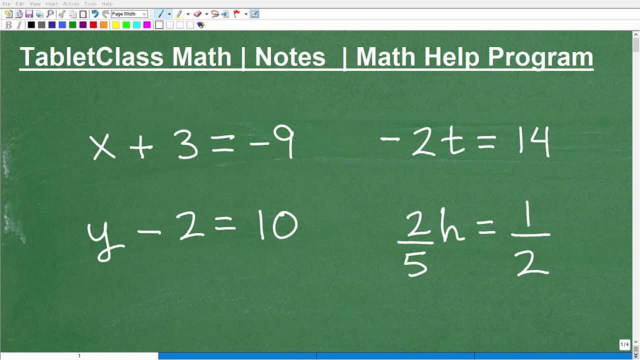 Okay, let's learn how to do these basic algebra equations. So hopefully, this is, you know, going to be a review for most of you out there, But if you're learning algebra- basic algebra- and you never, you know, studied this stuff or don't know how to solve these basic equations, I think this video is going to be a good little. you know it's going to be enough instruction for you to get this. However, you still want to obviously practice this in much more detail, But before you can solve more, you know basic algebra equations. I want to let you know that this video is going to be a good little. you know it's going to be enough instruction for you to get this. However, you still want to obviously practice this in much more detail. But before you can solve more, you know basic algebra equations. I want to let you know that this video is going to be a good little. you know it's going to be enough instruction for you to get this. However, you still want to obviously practice this. 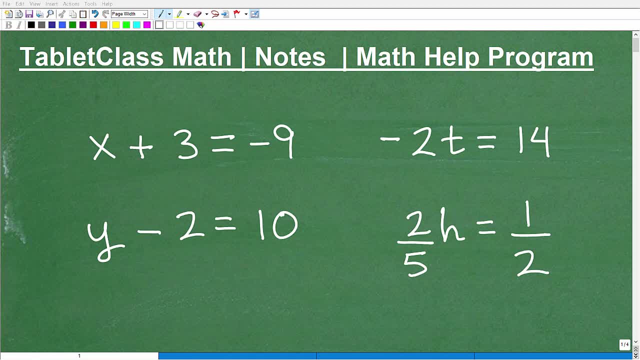 advanced equations in algebra, You got to know how to do the basic stuff. So we're going to focus on these problems here And I would also encourage you, if you think you know how to do the problems, kind of play along, pause the video and see if you can knock these problems out real quick. They should take you no more than you know literally one minute to do in total. All right if you know what you're doing, But we're going to get to each one here in a second. But first let me introduce myself. My name is John. I'm the founder of Tabit Class Math. 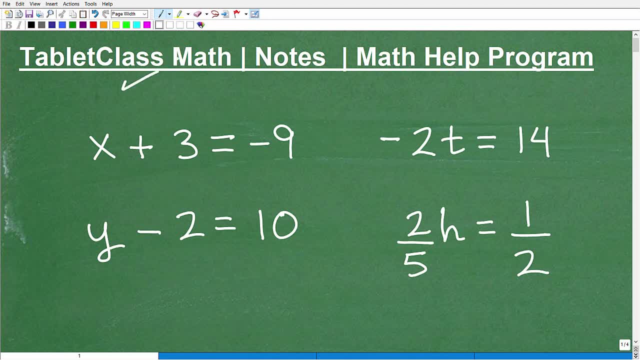 I'm also a middle and high school math teacher And over many years I've constructed just many, many online math classes. So if you're in need of math help- whether you need to take a full math course or some sort of supplemental assistance for the math class that you're taking right now- then you definitely want to check out my math help program. I'm going to leave a link to that in the description of this video. Also, if you need a pair of notes for something like this, you might want to check out my pre-algebra notes, But if you need a good reference set of reference notes for your math class, 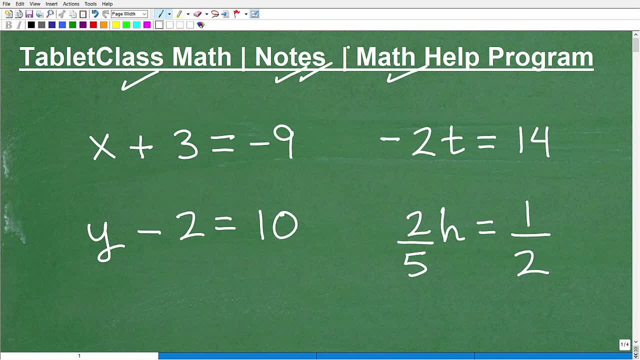 you can find the link to those notes underneath this video or in the description. Okay, so we got four problems here And let's just look at these things real quick. So we have an addition problem, we have a subtraction problem, then we have this is a multiplication situation. then we kind of have like a division situation. So we refer to these problems- okay, oftentimes are referred to as one step equations. all right, one step algebra equations, because 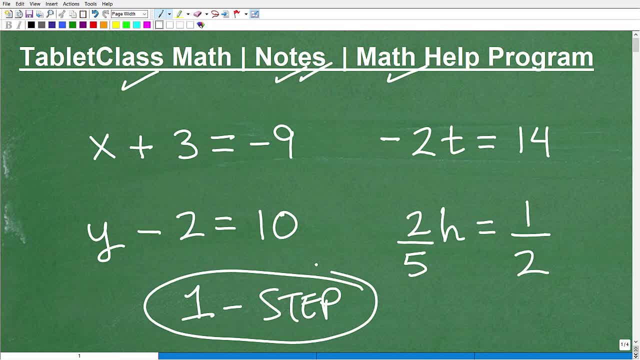 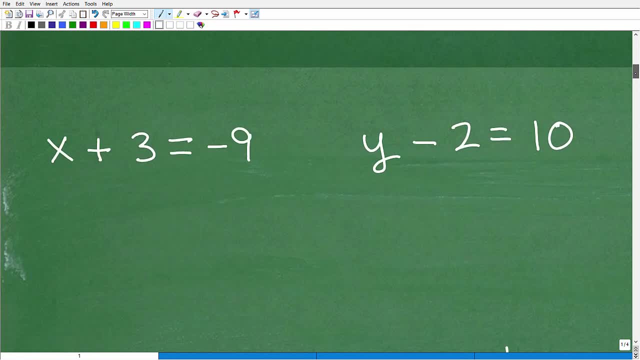 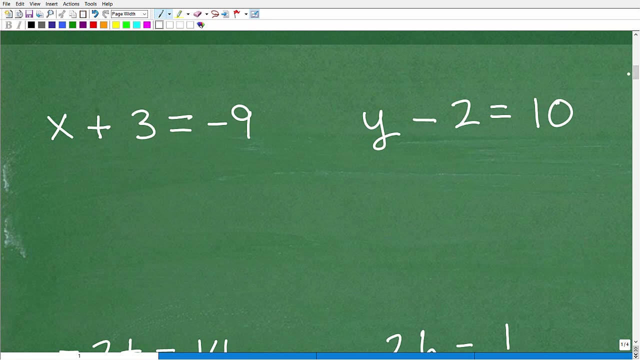 we're going to be able to solve these equations in one step, Okay, All right. So let's get to these problems now and emphasize some basic concept- concepts in algebra, All right. So the first thing is, if you you know, if you're watching this video, I'm assuming that you know how to work with positive and negative numbers. Okay, if you don't really know how to work with positive negative numbers right now, then you want to check out some of my other YouTube videos on the 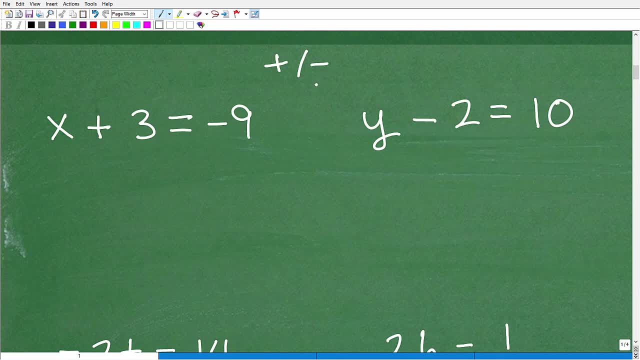 rules for positive and negative numbers. They're not difficult, but I'm going to be using them in our basic example here. Okay, All right. So here the main thing with algebra is the following: Let's just kind of use a little teeter totter, Okay, a little, a little swing here, right, A balance, of fulcrum, whatever you want to call it. kind of think of this as So, in equation, in algebra, we have all this stuff on one side, we have all this stuff on another side, And basically we're saying: 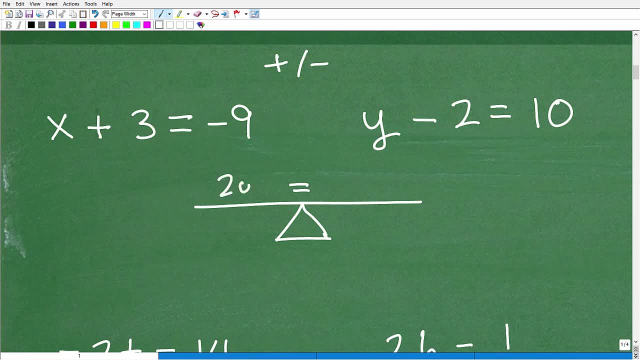 one side is equal to another side. So, like this side could be like 20 pounds And it's equal to this side. if it, if it's equal, right then the right hand side is 20 pounds, the left hand side. 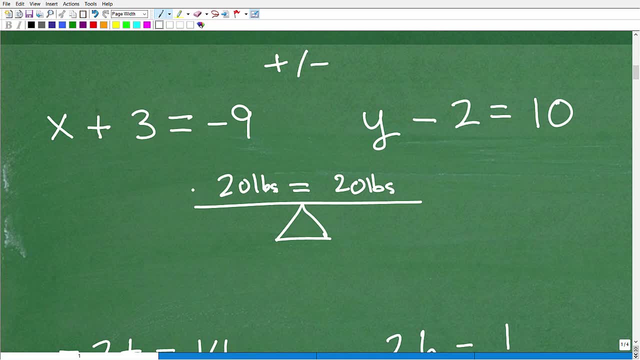 is always in balance. Okay, so let's say, I add five pounds to this side of the scale, Okay, what happens? Well, obviously it's going to tip like this: right, This is heavier, So to get it back in balance, I got to add another five pounds here. Okay, So in algebra, 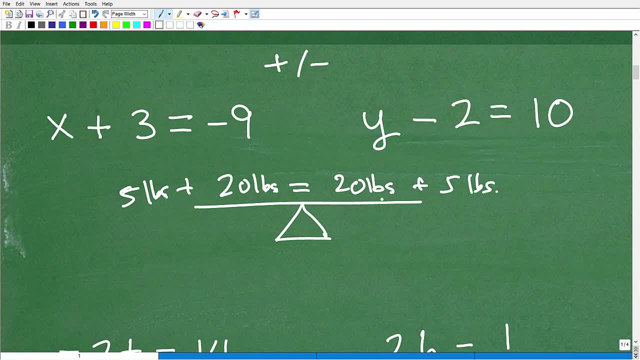 we need to keep the equation always in balance. always in balance, And that means conceptually, is the following right? Okay, kind of look at this way. So the main concept, the main rule of solving algebra equations is the following: whatever we do over here, 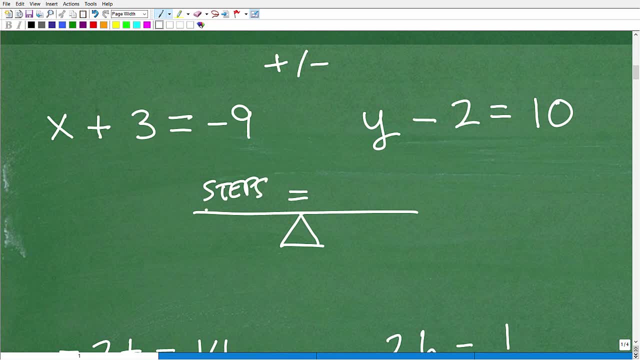 whatever steps we take on one side, okay, and I could take anything I want. It's like adding weight or taking weight off the scale. Whatever I do here, I have to do the exact same steps here, Okay. So whatever I do on one side of the equation, I could do whatever I want, as long as I do it. 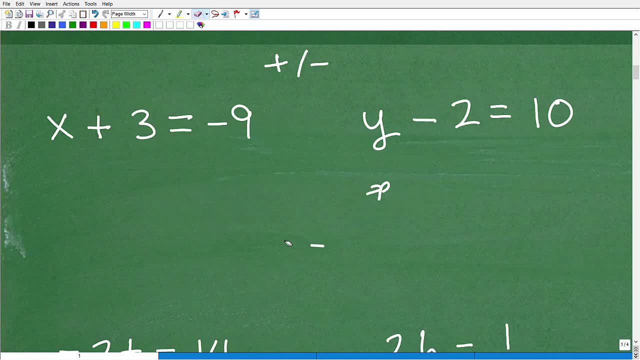 equally to the other side of the equation, And the objective- okay is to solve equations- is to get x equals okay, the variable by itself in some number. okay, and the variable could be x, y, t, z, it doesn't make a difference. Okay, All right. So, with that being said, let's get into 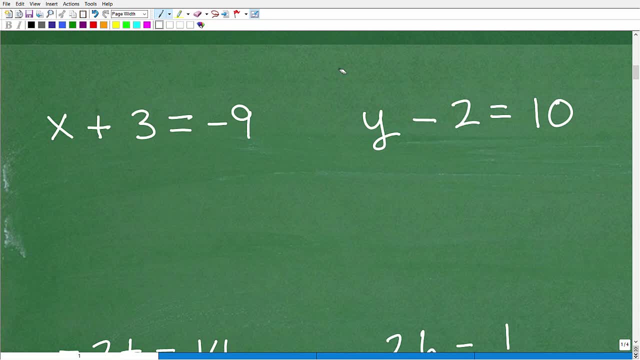 the basic mechanics of these one step equations. All right, We have: x plus three equals negative nine. So I want to get: x is equal to okay. x is equal to itself. So how can I get? x is equal to itself, but I got a plus three here? Well, we can be like: 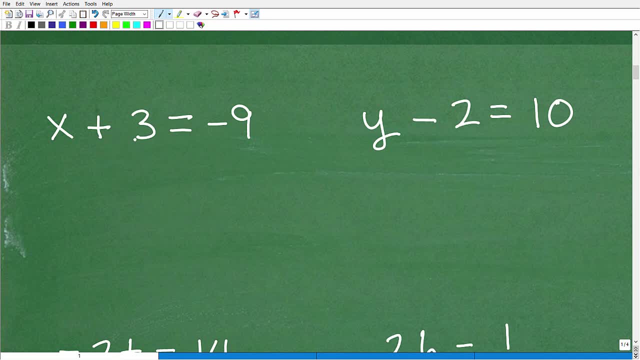 let's just get rid of this three. Let's just get rid of it Like, hey, three, we don't want you here. I hate to kind of say it that way, But let's get rid of the three. How do I get rid of a? 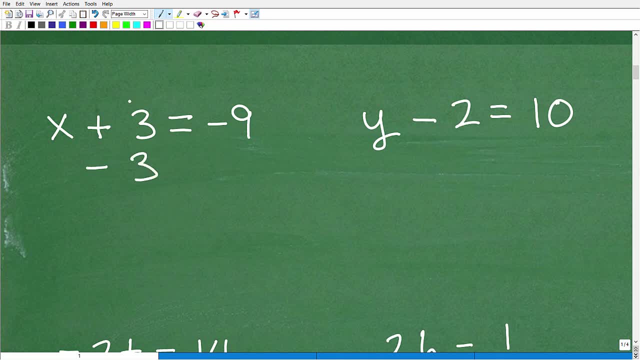 positive three. How about we just subtract a three? Okay, if I got a positive three, I can get rid of subtracting a three, No problem, right. However, remember the rule: whatever I do to one side of the equation, I have to do the exact same thing to the other side. All right, So the way I'm writing. 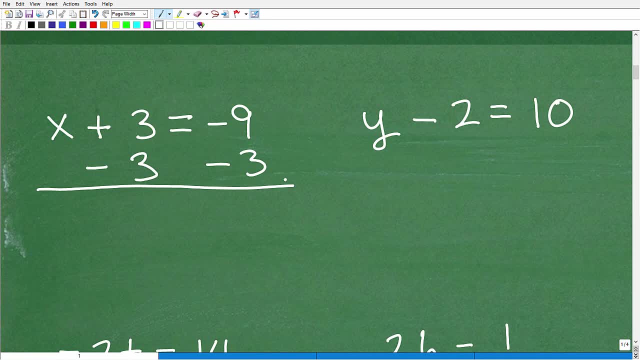 this is the way you should write it as well. Okay, so we're going to draw a little line like this. So what I'm doing in essence- okay in our little scale- is I'm adding a negative three to both sides. All right, I'm not damaging the equation, I'm keeping it in balance, But it's going to help. 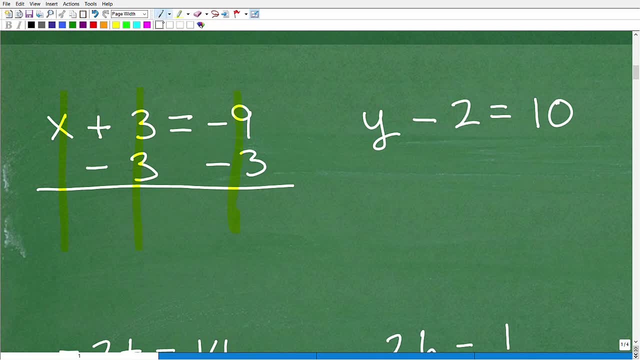 Now, when you write an equation like that, you kind of want to add down in a column manner: So x plus nothing is what Just x. All right, we'll write that x right here, Because positive three plus a negative three or three minus three is what Zero. I don't need to write a zero there, Okay, it's just. 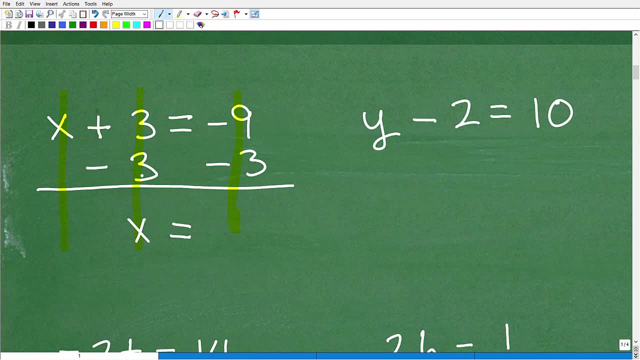 implied It's these. I got rid of the three over here on this side, And then negative nine plus negative three is a negative 12.. Okay, And that is my solution. That's it. It took me one step. The step that I took was to add negative three to both sides of the equation. All right, so 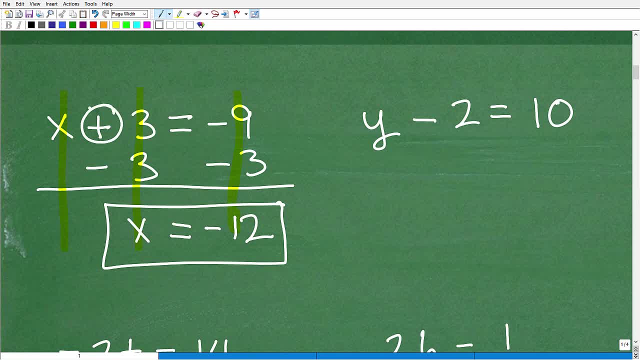 if you kind of understanding. okay, for to get rid of this positive three, I had to use the opposite operation- negative. Well then, let's kind of go to our next problem and see if we can apply that same technique over here, because it's pretty similar, right? 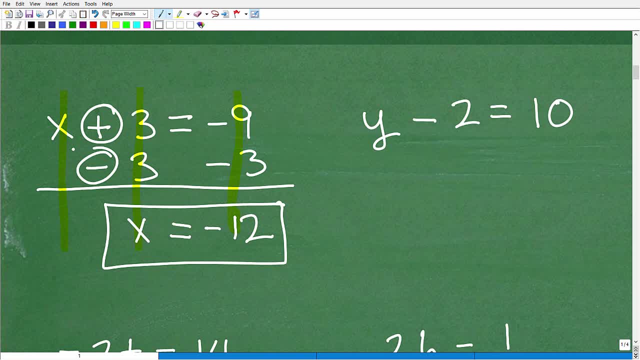 All right, anytime you think you could do these problems, you should just pause the video and do it. But let's get into: y minus two equals 10.. All right, well, I want the y by itself, So I can get y by itself. Well, we got to get. we have to get rid of this negative two. 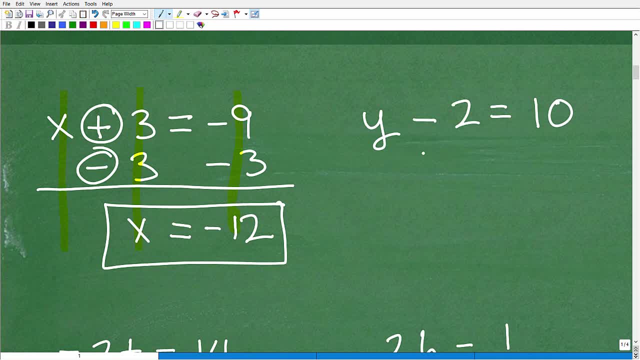 next to the y. We're like: hey, sorry, we're going to have to get rid of you. So how do I get rid of that negative two? Well, how about we add a two, a positive two, okay, to it. So I got negative two. 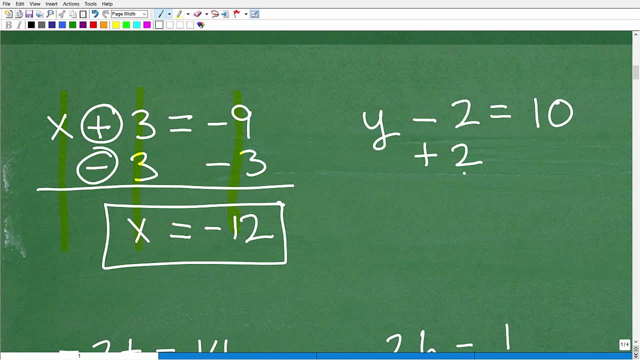 we'll add a positive two to it. it's going to make it vanish, But I also got to do the exact same thing on the other side. That is the main rule of algebra, right? So I want to add down in a column manner. I'm going to get: y is equal to negative two plus two. 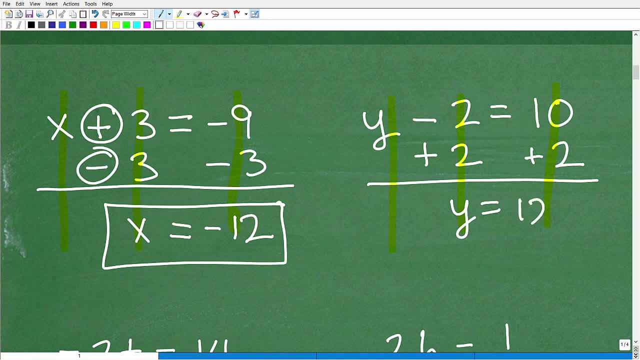 zero, it vanishes, And I have 10 plus two, which is 12.. And there you go. Okay, so what was the one step? The one step was just adding two to both sides of the equation. But notice the pattern. 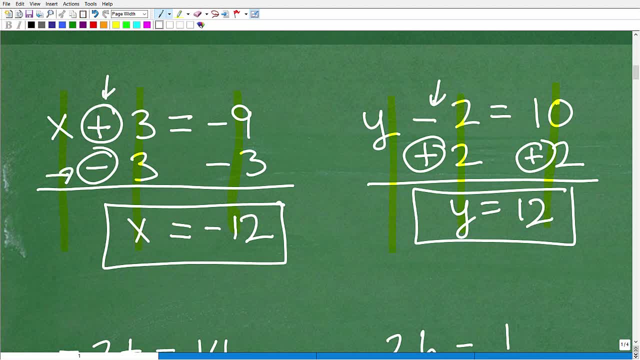 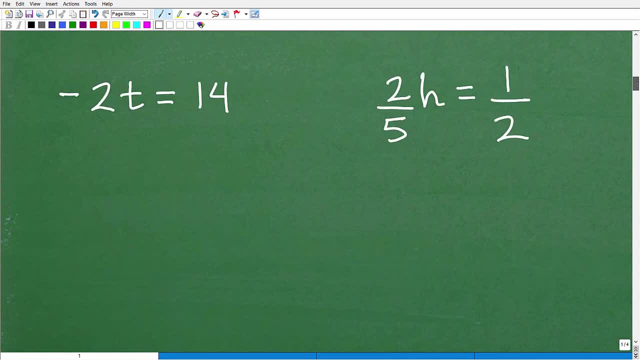 here: When it was negative, I had to add, When it was addition, I had to use subtraction. Okay, this is the kind of concept, another concept of solving equations, algebra called like inverse operations, we call it, but we don't need to get into all that fancy. 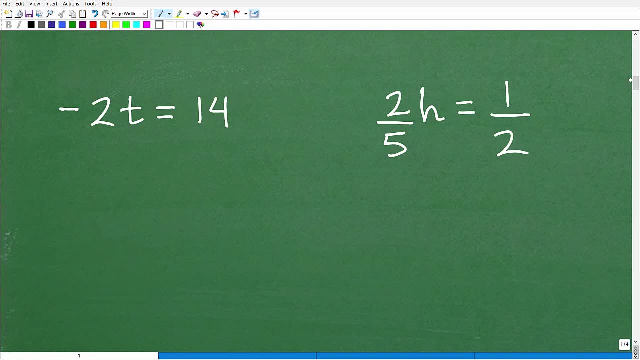 nomenclature. Let's get into our last two problems. Okay, this one is what? What operation is this saying? This is negative two times t, This is multiplication, right? So when we have multiplication, what would? be well, let me go back this way, When we had addition. 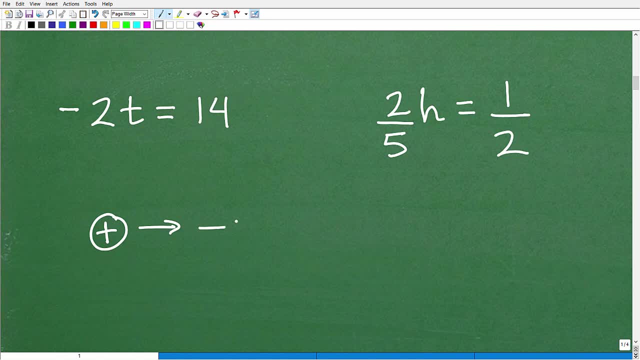 its inverse operation was subtraction, right? Well, we just- I'm talking about the answer, as we just did. When I have subtraction, its inverse operation is addition. So, if I have multiplication, what do you think its inverse is going to be? Yes, you guessed it: division. 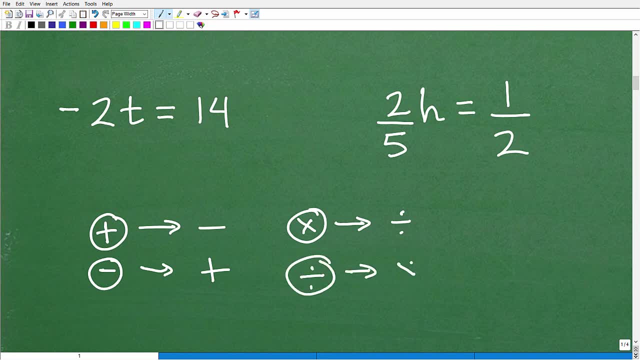 And let's just go ahead and do it here. If I have division, what's its inverse multiplication? Okay, so here I have negative. two times t equals 14.. I want to get to t by itself. So it's multiplication. So the way to get t by itself is: 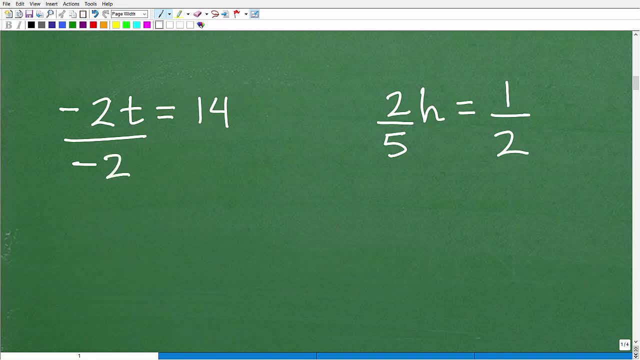 I could divide both sides of the equation. I could divide this side by negative two, okay, Because anything divided by itself okay is going to be just one, a nice positive one, right? So if I take negative two and I want to get rid of that, in front of the t I'm like: 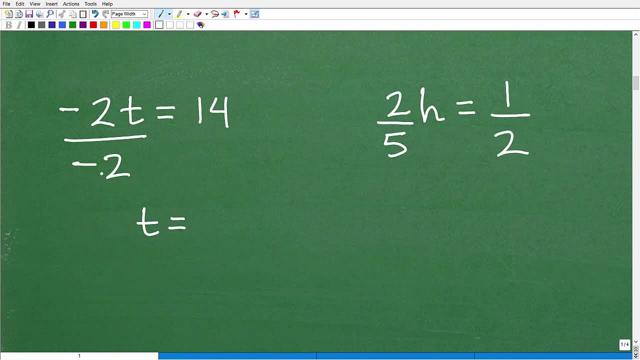 I just want the t. I don't want the negative two part. If I divide that by itself- negative two- I get a positive one t. But again, the main rule of algebra is: whatever I do on one side of the equation I got to do to the other. So 14 divided by: 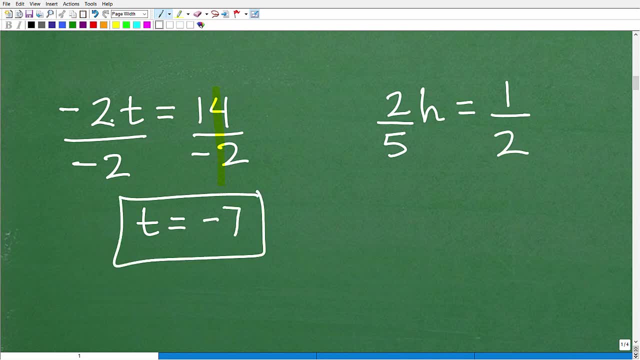 negative two is going to be negative seven, all right. So here I had multiplication, but I used division to solve this one-step equation, All right. so I kind of left the best for last. This one kind of confuses students, So I'm going to give you the easiest way to think of how to do. 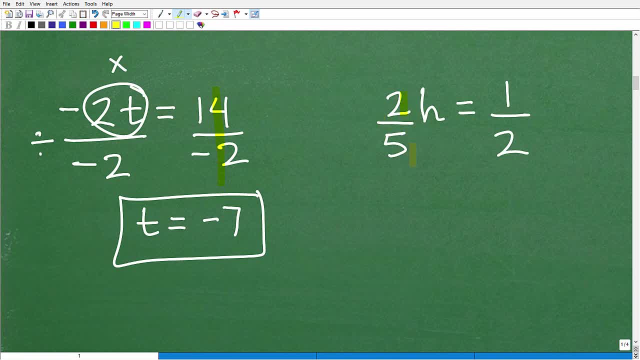 this All right. so here we have two-fifths. Okay, it looks like division. I could kind of look at this this way. An equivalent way of writing this problem would be: two h over five equals one-half. Okay, this means the same thing. Okay, so we're kind of dividing. 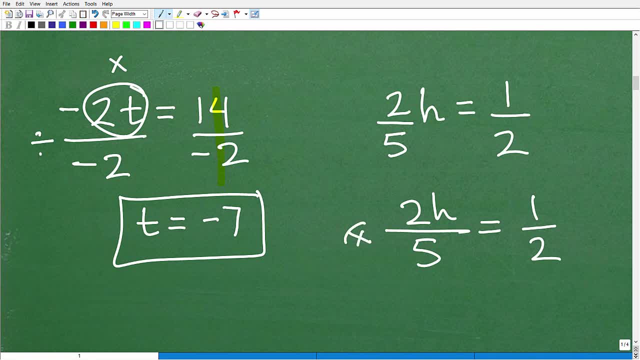 So this is like a division scenario. So we're like, okay, we're going to use multiplication, We are going to use multiplication, but I'm going to show you the easiest way to approach these problems. So this one is: two-fifths times h, equals one-half. So how do I solve a scenario? 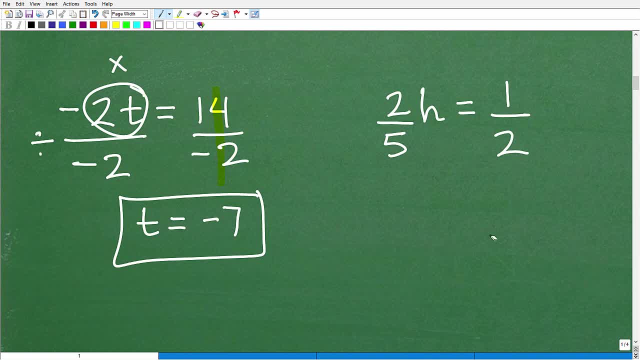 here I want: h is equal to itself. Here's the deal. okay, Anytime you have two-fifths, you have a fraction in front of a variable, just like this. Okay, all you have to do is flip this guy upside down. Okay, which is what? Five-halves, All right. and when I multiply five-halves times? 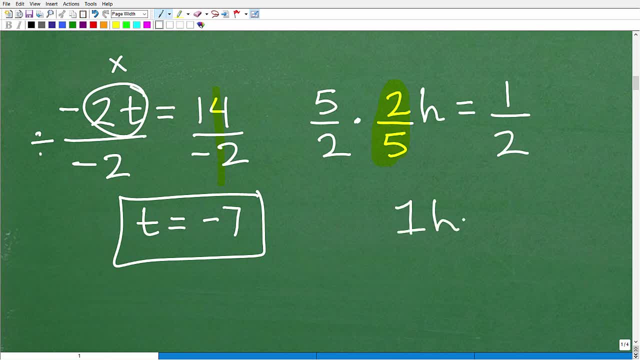 two-fifths. I'm going to get one h or just h. Okay, that's what I want, right? The objective is just to get h by itself. All right, and I could do that. I got this two-fifths in front of here. 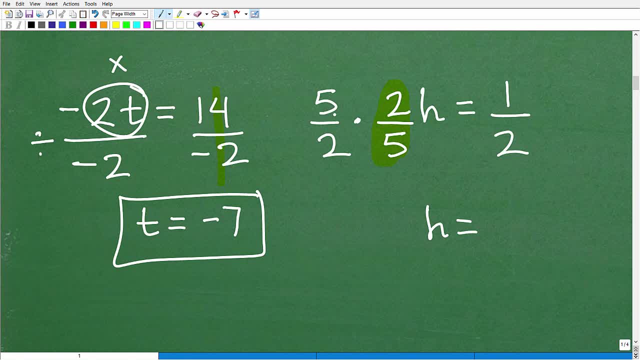 I'm like: how do I get rid of you? I multiply it by what we call its reciprocal. So that's going to be five over two, because when I multiply across I'm going to get ten over ten, or one okay, Or one h, or just h. We don't write. 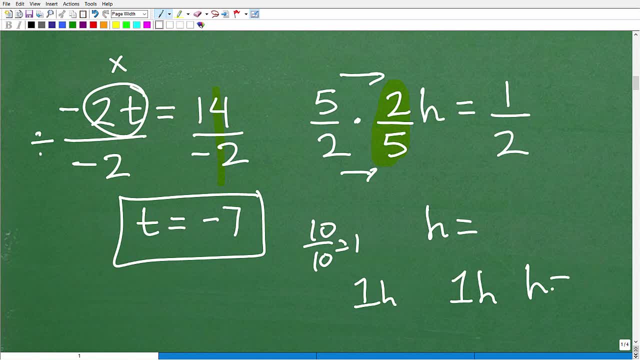 like one h, We'll just write h, okay. This means there is a one in front of the h, but we never really write the one. Okay, but what's the deal here? Well, the deal is what I multiplied the left-hand side by five-halves, so I have to do the same thing. 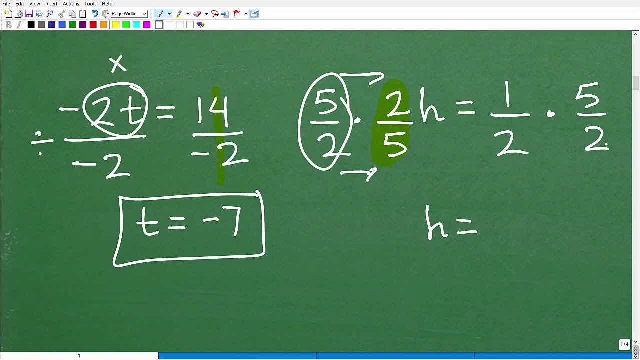 on this side. You got to always be fair. all right in algebra, Okay. so now, once I figure this out, I'll have my answer. Okay, so five-halves times two-fifths is h. We already talked about that. 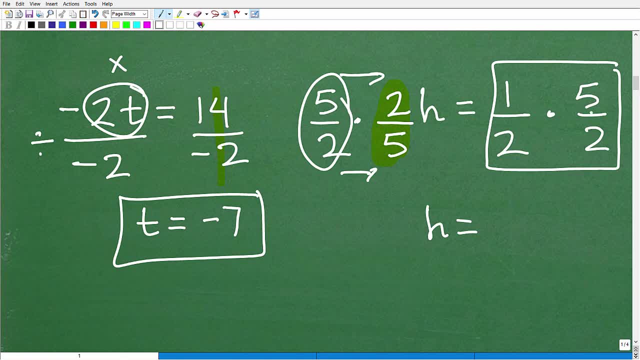 one h. So one-half times five-halves is going to be five-fourths, right? We just multiply across and that's it We are done. Yay, So we get our little happy face, our little stars, you know. 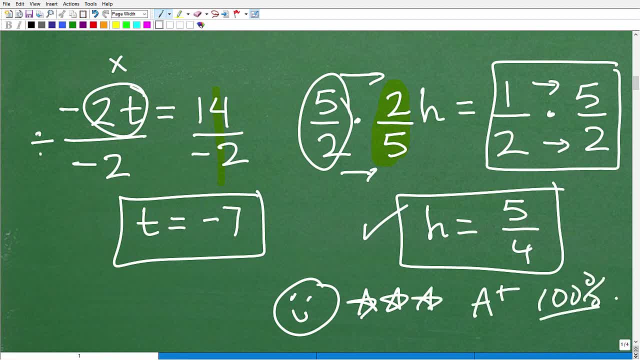 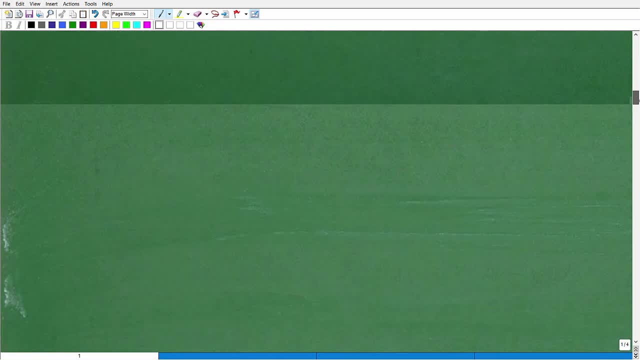 or a hundred percent, That's the good stuff, right? And you're like: oh man, I aced that quiz, okay. So here's the thing: Before you can understand complicated, you know equations like I don't know. let's just say: write something like this: 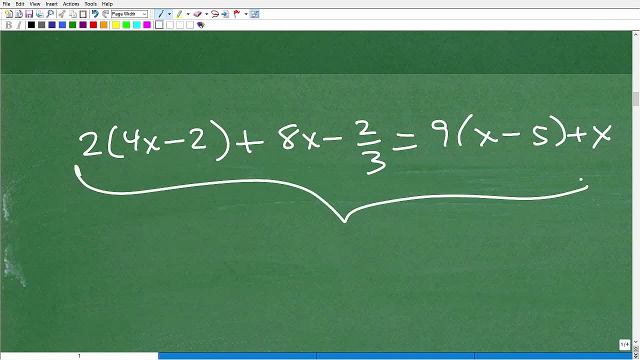 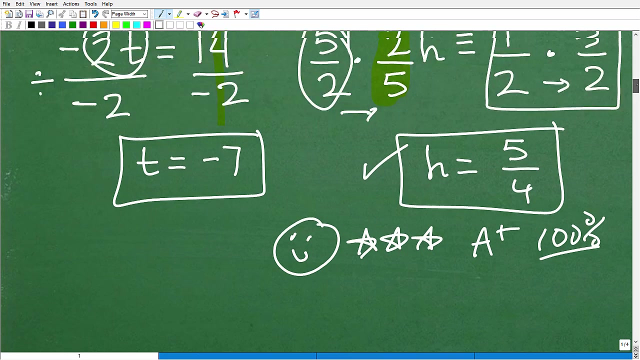 So, before you can understand how to solve an equation like this in algebra, okay, we have to. this is what we call a multi-step. multi-step equation. It just requires multiple steps to do. all right, But those individual steps, the again multiple steps, but each step, okay, effectively is the. 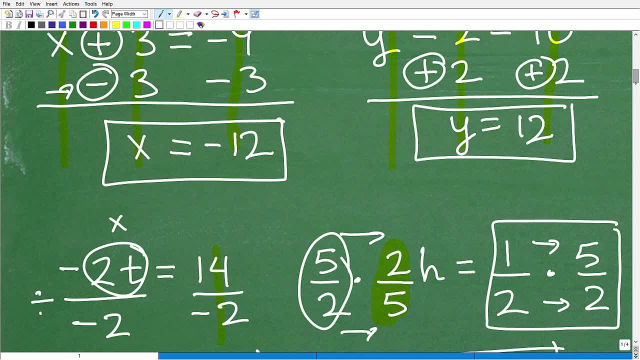 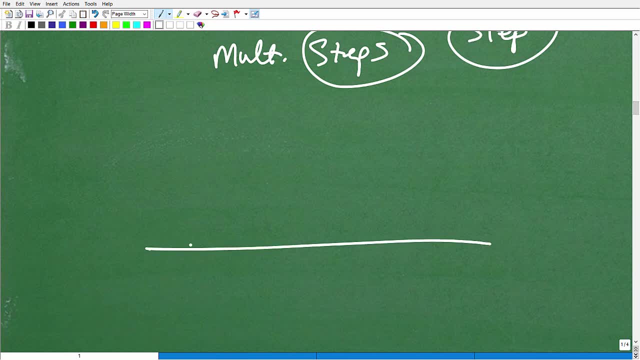 steps that I just went over. These are the four primary steps that you need to understand. So once you understand how to do that, then you can, you can, you know- climb as high as you want in algebra. It's like walking up. you know actual steps. right, I'm kind of these are some messed up. 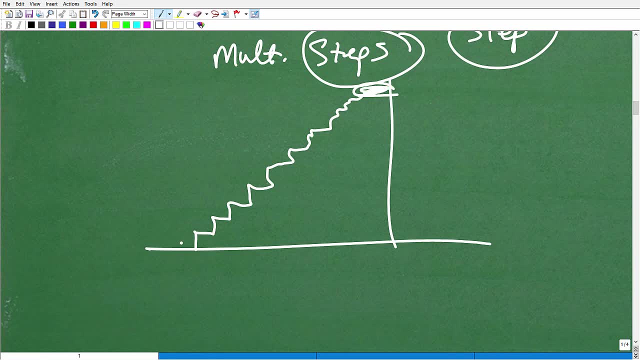 steps, but you kind of get the idea. If I want to get to this right here, as long as I know how to go from this step, oh, and just climb another step. well, I'm just repeating myself, right, I'm. 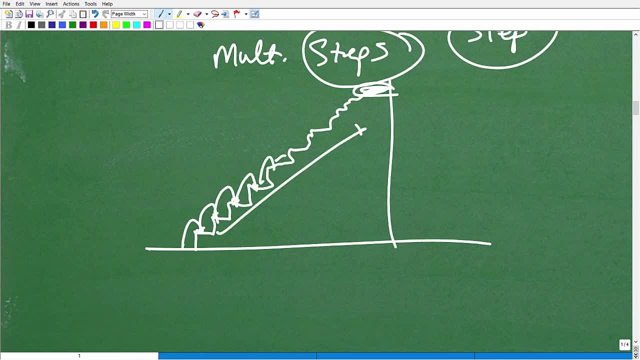 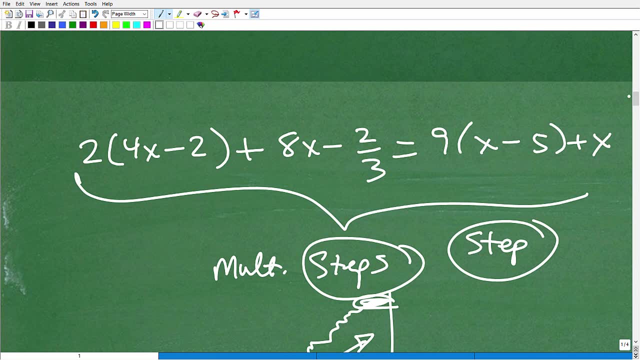